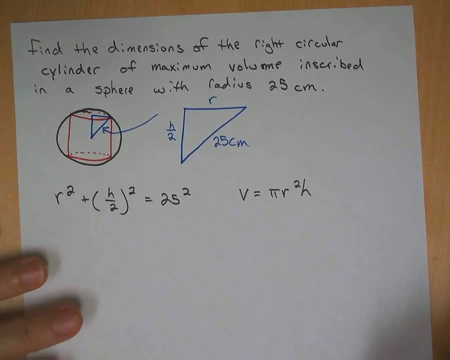 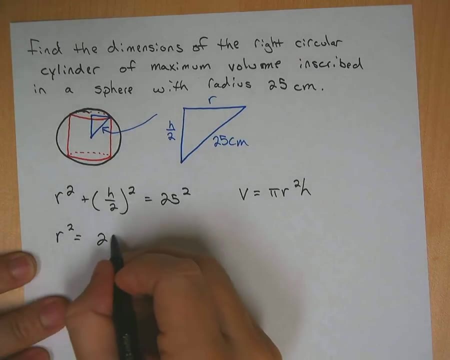 Instead of the r and the h, we want to get rid of one or the other. Okay, so, in order to do this, I'm going to solve this equation for r. So we get: r squared equals 25 squared minus h over 2 squared. 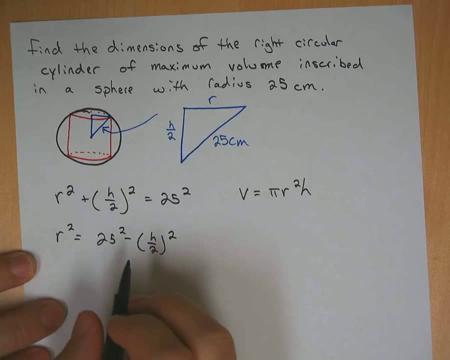 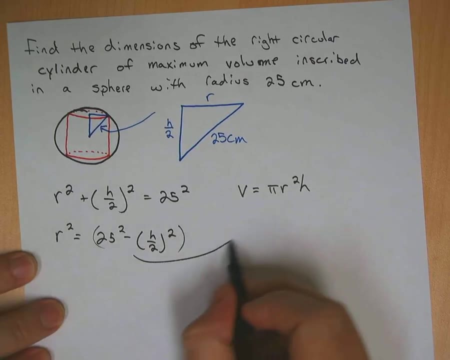 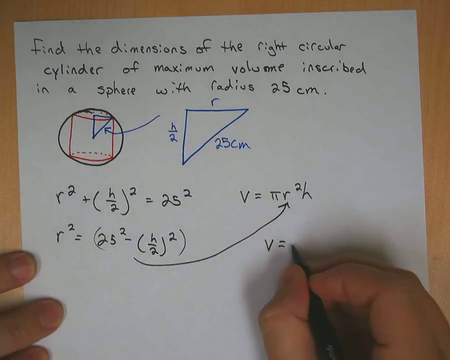 Okay, and then I can take, I can take the I can take the volume here formula and I can plug in right there in place of r squared, because that's what this is. Okay, so I would get: v is equal to pi. 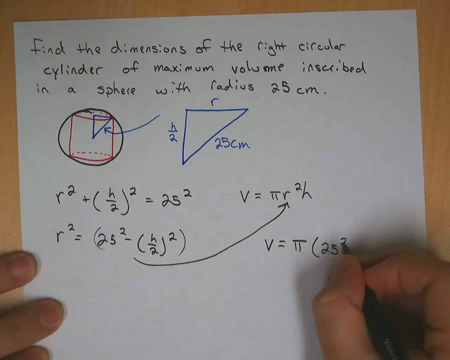 Now I'll plug in here. I get 25 squared minus h over 2 squared h. Okay, clean that up a little bit, I'll get. volume is equal to pi times 25 squared h minus h cubed over 4.. 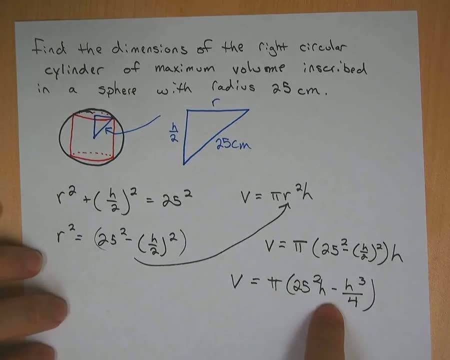 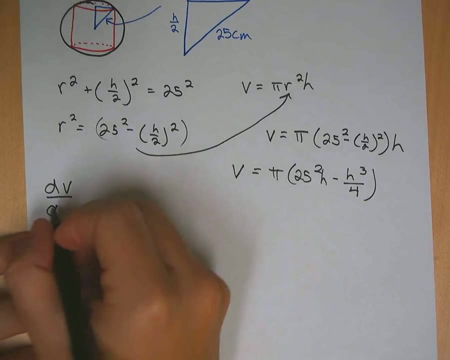 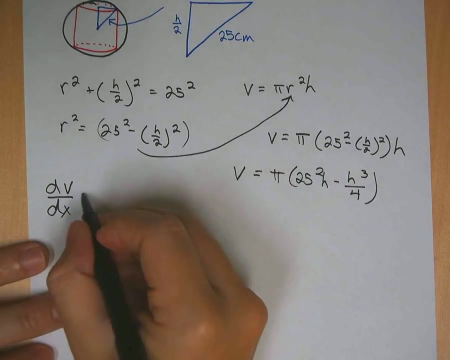 Okay, so I've got this in terms of just h instead of h and r. now, Okay, I'm going to go ahead and take that derivative, dv, dvd- We'll just say dvdx. Okay, so We take this derivative and that's going to be pi. 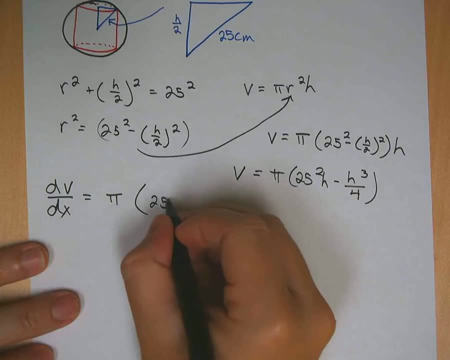 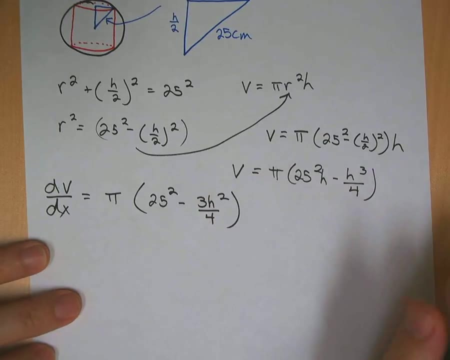 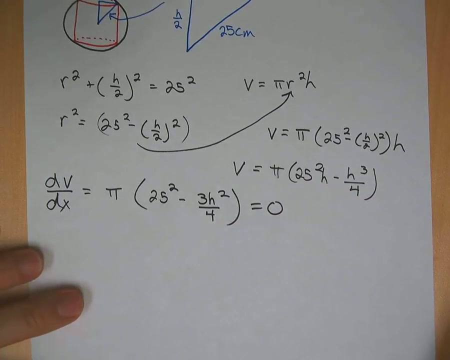 It's constant on the outside: 25 squared, the h goes away, minus 3h squared over 4.. Okay, To find the critical numbers, we set this derivative equal to 0.. Okay, so we solve this thing down. 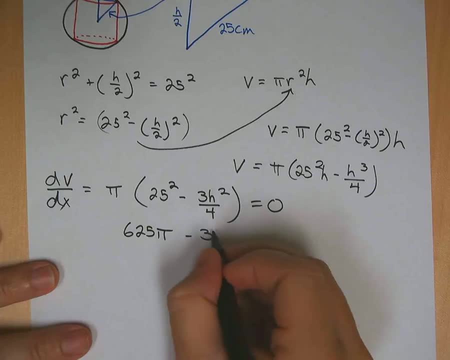 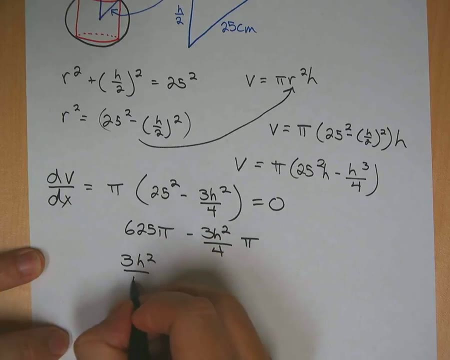 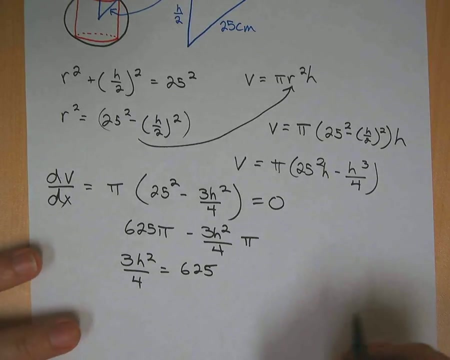 We get 625 pi minus 3h squared over 4 pi. That will give us 3h squared over 4 equals 625.. The pi's will cancel out when we move this over. So we'll get, We solve that over and we get: h is approximately equal to 28.87..